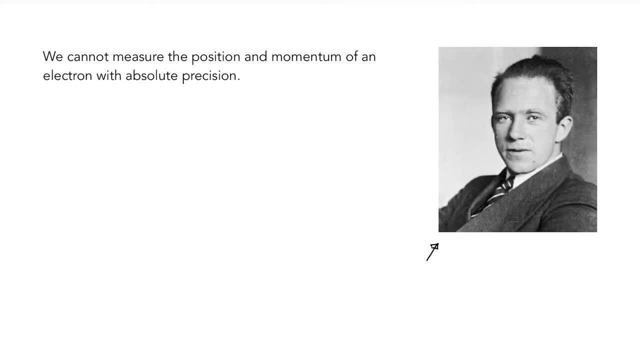 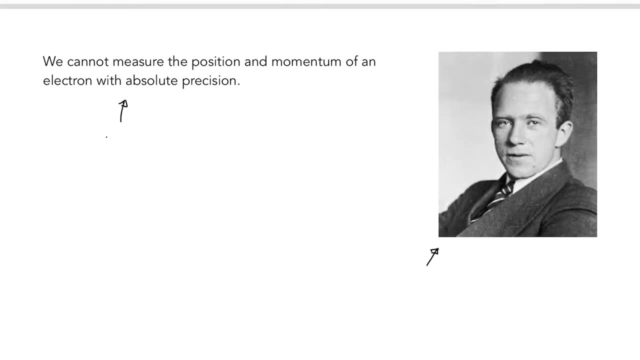 We cannot know the precise position and momentum simultaneously, And this is known as the Heisenberg uncertainty principle. That was a Heisenberg uncertainty principle. So if we can't know the precise location of an electron in an atom, it would be more accurate to 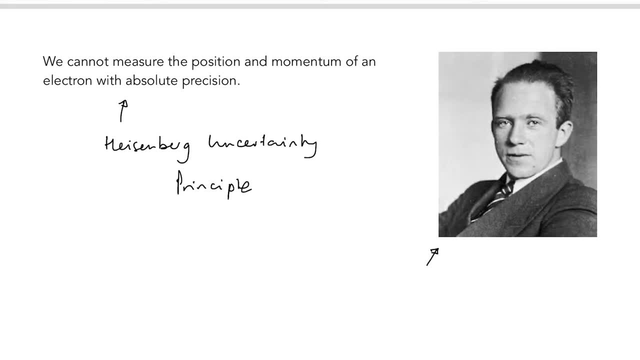 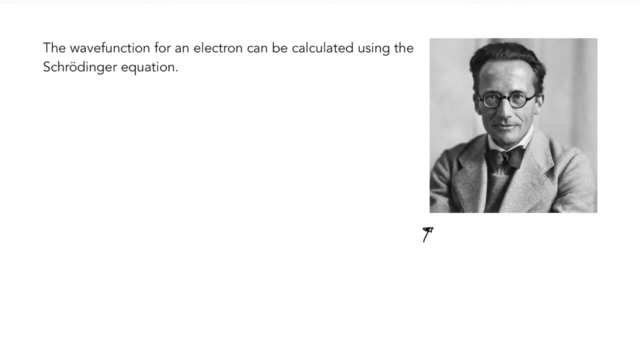 to consider the probability of an electron being in a certain volume of space. So we're thinking about electrons' behavior in terms of waves more than particles, And this is a big departure from what we were looking at at GCSE. So this gentleman here, Owen Schrodinger, incorporated the ideas of 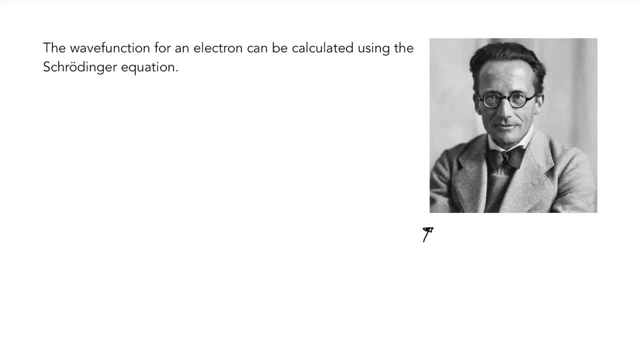 both Heisenberg and de Broglie into a mathematical model, And in this mathematical model he introduces us to the concept of a wave function. Now the wave function for an electron can be calculated by solving the Schrodinger equation, which is really complicated and way beyond the 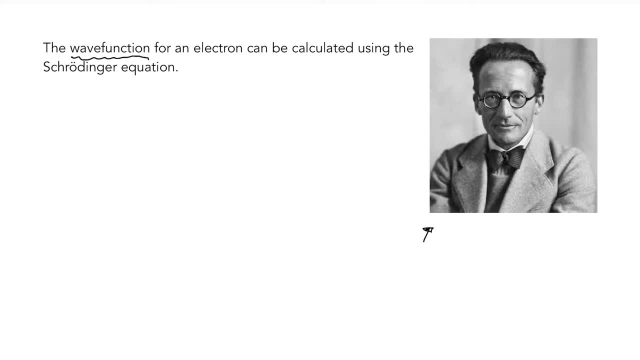 scope of this little video. But when you solve this Schrodinger equation and you calculate the function electron, It contains detailed information on the behavior of an electron. That was the good news. The bad news, Unfortunately, this is totally abstract and it's not useful. And the equation 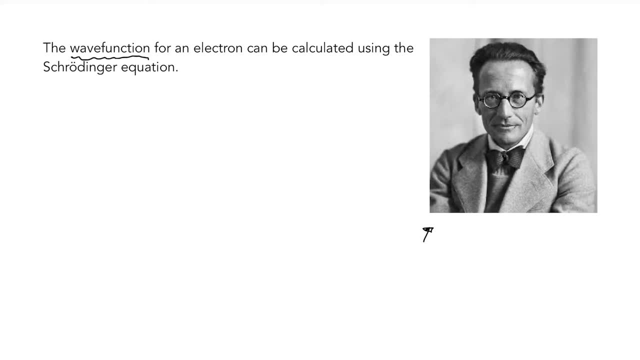 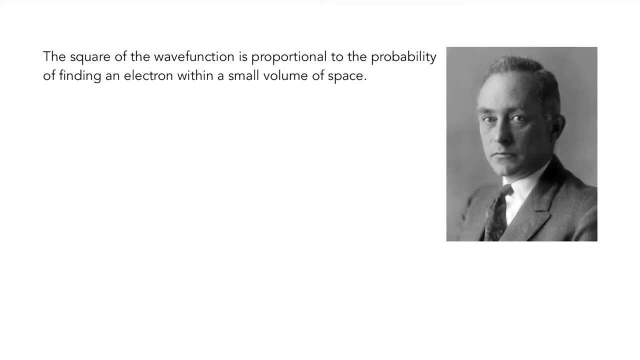 can only be sold for a hydrogen atom, which is also not very useful. However, luckily for us, Max Born came along and he suggested that the square of the wave function is proportional to the probability of finding an electron within a small volume of space. And the electrons are. 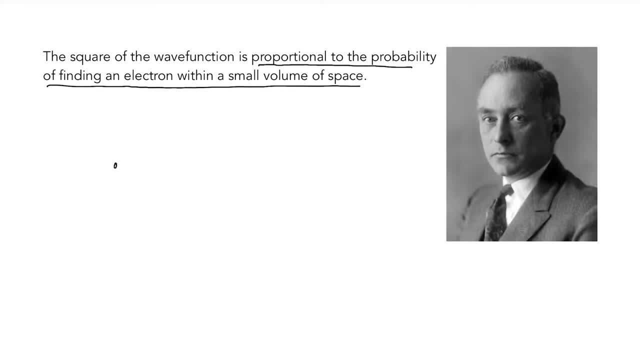 spread throughout this volume of space. So we're not thinking electrons here are particles. They're not in fixed orbits, like the Bohr model of the atom that we used at GCSE would suggest. We are now thinking that electrons behaving as waves are spread out through a fixed 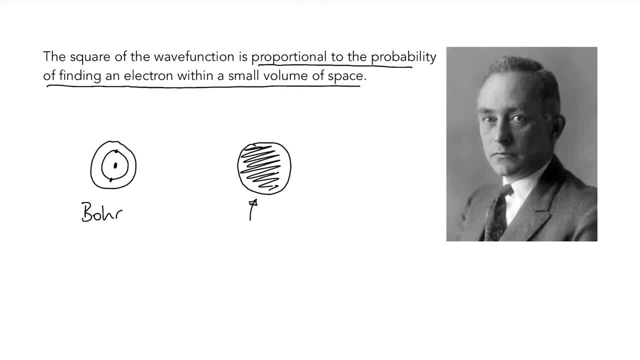 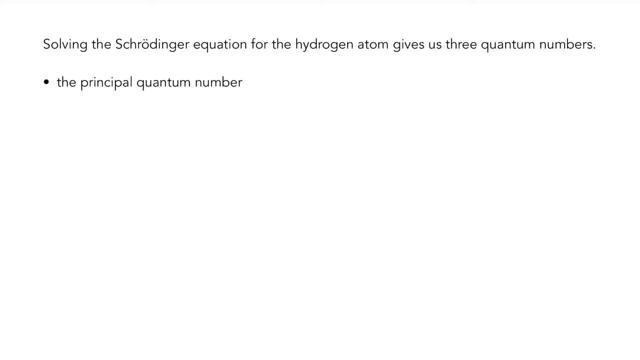 volume, And that fixed volume of space is our atomic orbital. So the Schrodinger equation can be solved for the hydrogen atom, And when you do that it gives us three quantum numbers. The first quantum number is called the principal quantum number and it's given the symbol n And it shows that the electron in our 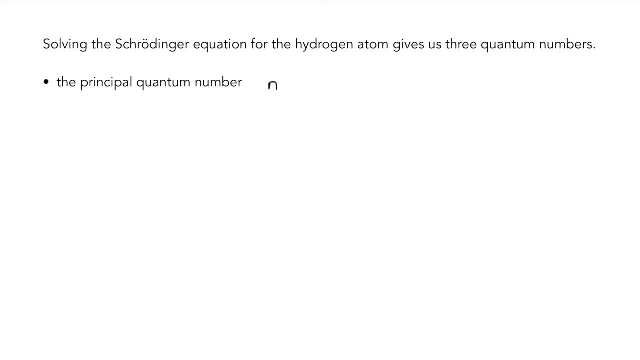 atom can only possess certain energies And these correspond exactly to the energy levels we see in atomic spectra, which is very nice indeed. So each energy level is referred to by its principal quantum number and it's an integer. So we can have the first energy level, the second, the third. 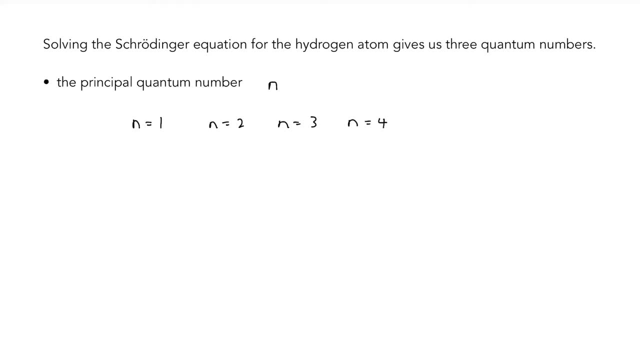 the fourth. So when we looked at atomic absorption emission spectroscopy, these were the labels that we used for our energy levels. The next two quantum numbers that emerge help to describe the properties of a particular atomic orbital. The secondary quantum number it's also known as the angular or sometimes the orbital. 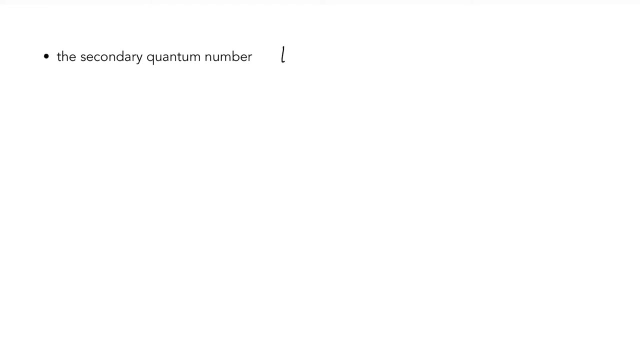 quantum number and it's given the symbol l. That's an l, not a number one, And it can be any whole number, from zero to n minus one, n being the principal quantum number or our energy level. The good news is that the quantum numbers that emerge are not the properties of a particular atomic orbital. 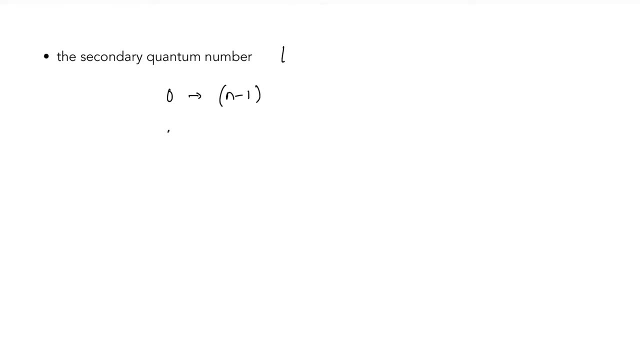 Notice that, as far as atoms and chemistry are concerned, that the only values of l that we're interested in are naught one, two and three, And I'm going to come back to this in a little bit more detail in a second. And then we have the magnetic quantum number. It's given the symbol ml. 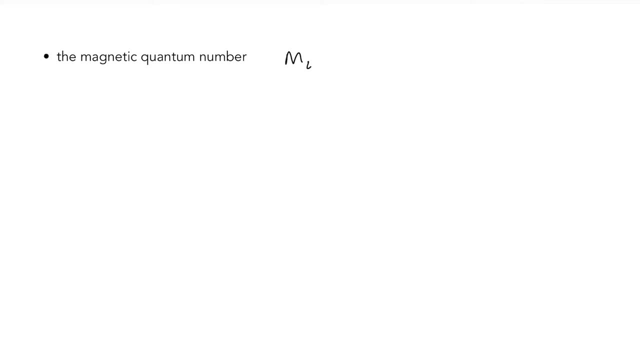 You need to write that quite carefully And it can have any value, from minus l to plus l. And be very careful that when I write that it doesn't look like minus one to plus one. So minus l to plus l. So our three quantum numbers. we've got the principal quantum number, which is giving us 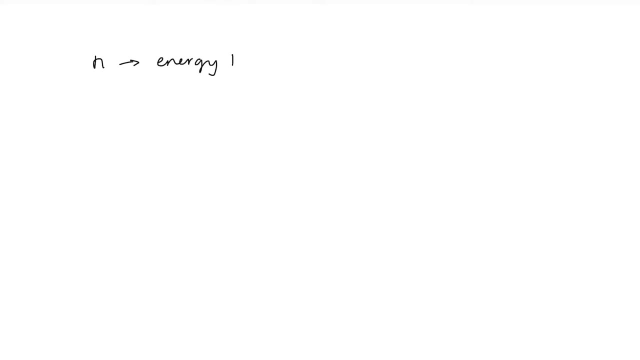 the energy of our orbital, ie which energy level this orbital is existing in Our secondary quantum number, l, which is telling us about the shape of the orbital. So let's have a look at this in a bit more detail. The shapes of these orbitals are given letters, And this is something you should be familiar with. 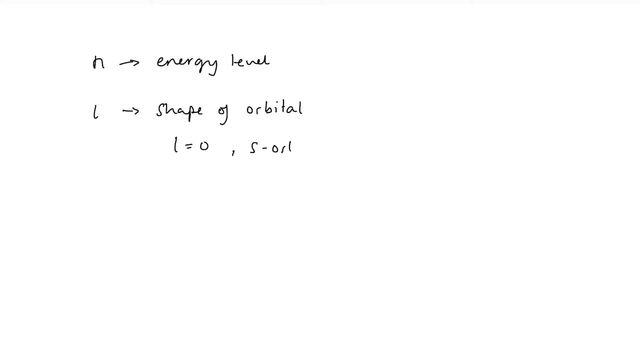 When l equals zero, we've got an s orbital. When l equals one, we've got a p orbital. When l equals two, we've got a d orbital, And when l equals three, we've got an f orbital. And then our third quantum number, m, gives us the orientation of that orbital in 3D. 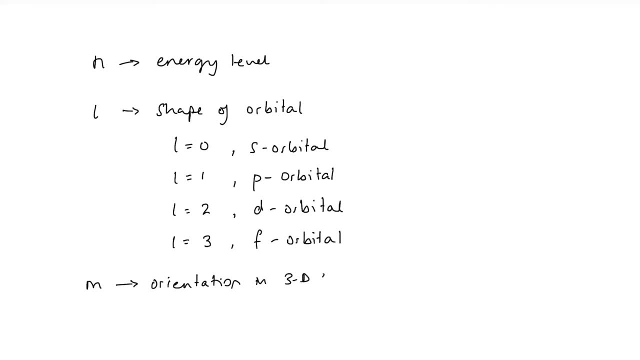 space Orientation in 3D space And in the third shape of L you put s power in that fürs. When l equals one, we've got the se говорил Thatículows side, And when l equals four, we've got all the others. So it's basically a 3d space. 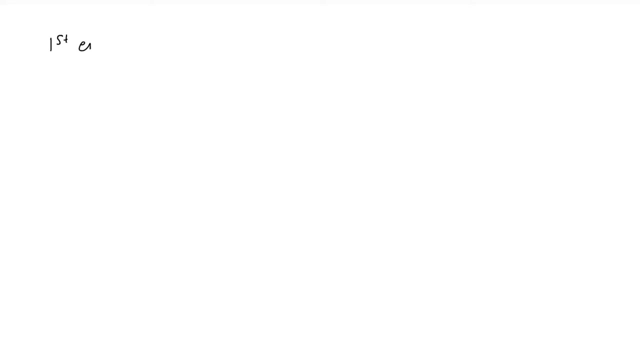 Or the � equals n Kubicki space. Whatever I type in here. Just add n equals M. And then our third quantum number, m, gives us the orientation of that orbital in 3D space. Orientation in 3D space. Our first energy level. First energy level, We know that n equals one. The first equation would be intercalating from Y equals one. to sew Is aaki thought that N equals one, But we lists a combination when step two is an evaluation of respect and 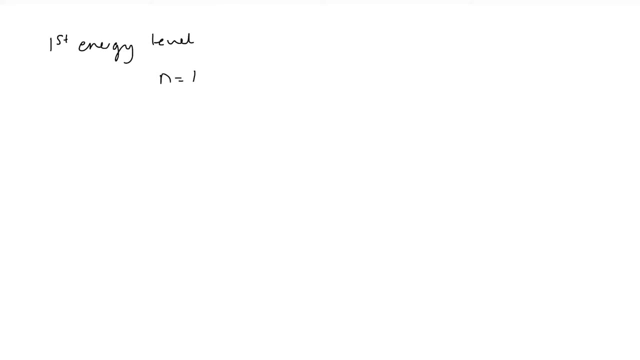 We know that N equals 1.. L can either be 0 or it goes up to as far as N minus 1.. Well, 1 minus 1 is 0. So in this case, L can only be 0. And ML is also 0. So that is telling me that. 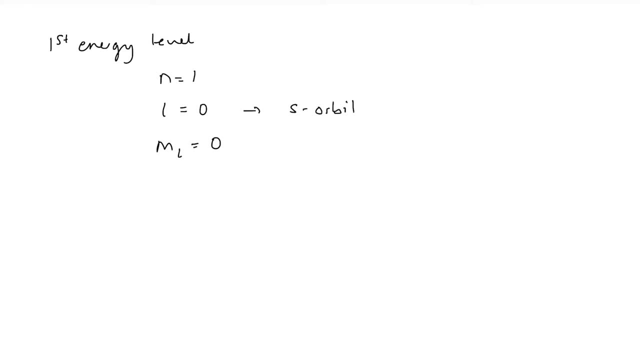 we have got an s orbital in our first energy level. So we might know that, as the 1s orbital And the orientation in 3D space is 0. We know that because the s orbital turns out to be spherical, It doesn't have a direction. Second energy level: Well, N equals 2.. L can equal. 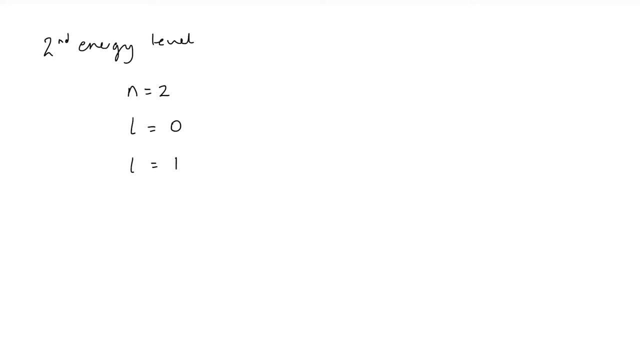 0. So that is telling me that we have got an s orbital in our first energy level, So we might know 0.. Or it can equal 1.. If it equals 0,, then I know that ML also equals 0,, which corresponds to our 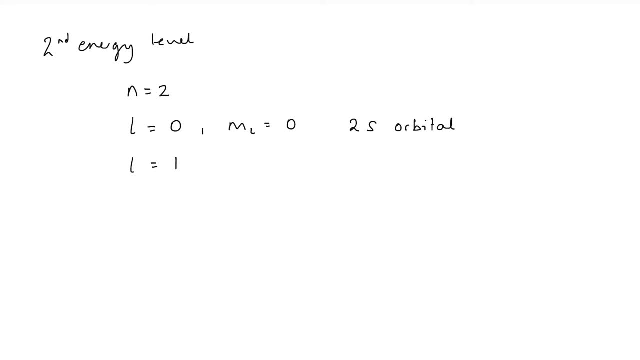 2s orbital Where L equals 1,. we have got a 2p orbital And ML can either be minus 1,, 0, or plus 1.. What does that mean? It means that we have got 3p orbitals, each with a different orientation. 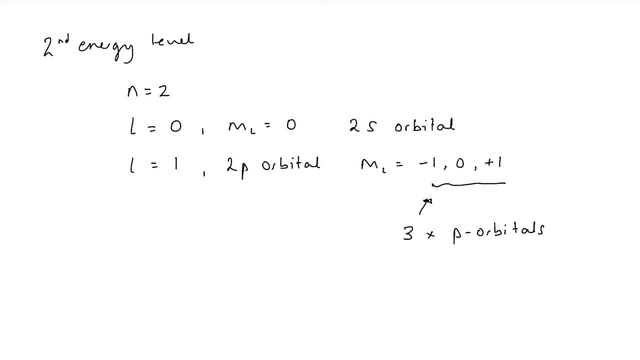 in 3D space. So let's take a look at the third energy level. Every time we move up an energy level, we have got more atomic orbitals available to us. N equals 3.. L can equal 0.. It can equal 1.. 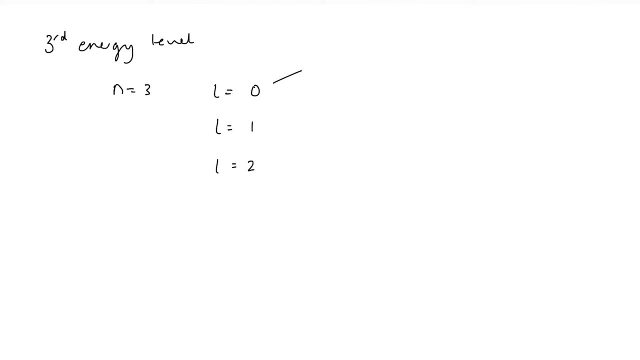 And it can equal 2.. We would then then have a Vega program telling us: BL equals 1.. ONE of these có perlán a 3s orbital, And this time Bloom will say: L equals 2.. When it equals 0,, well, that is telling me that ML is also 0, and this corresponds to my 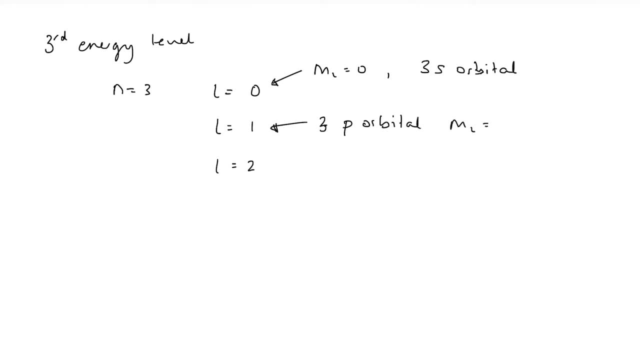 3s orbital When L equals 1,. we've got our 2p orbital, So that's my 2,3, even my 3p orbital, And once again, ML can be minus 1,, 0, or plus 1.. So I have got. 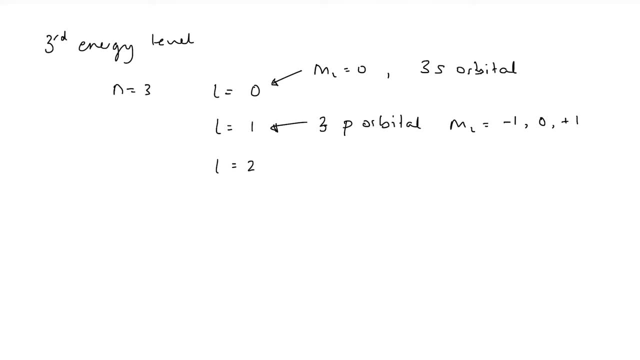 three 3p orbitals. When l equals 2, that tells me that I've got a d orbital. So it's my 3d orbital because it's in energy level 3.. And my magnetic quantum number can have values from minus 2,. 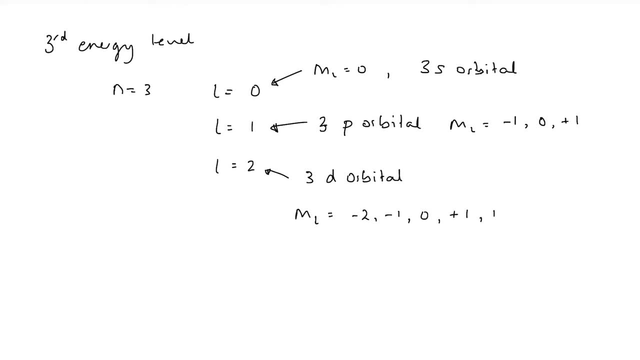 minus 1, 0, plus 1, plus 2.. So what does that tell me? It tells me that I'm going to have five different d orbitals, each with a different orientation in 3d space. So, putting all that together, our wave function is also giving us information about the shape. 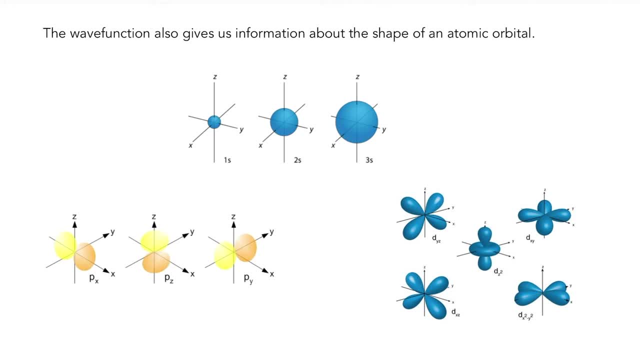 of an atomic orbital. Now the shape is shown by drawing a boundary surface. This is what we've got here, our boundary surface, And it represents the probability of containing a 3d orbital, About 95% of the wave function. Now, remember that we are thinking about electrons in terms 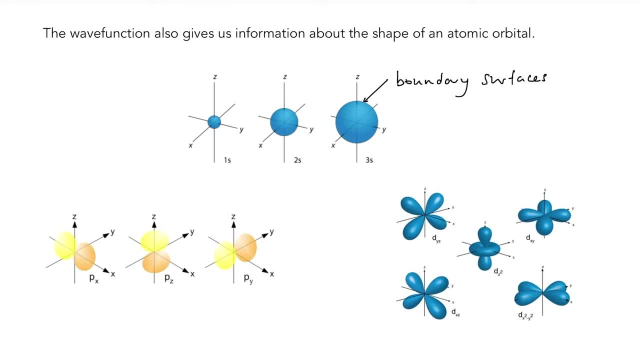 of waves that are spread out through a specific volume in space. So what we're saying here is that if we take my 2s orbital, then my electrons in that 2s orbital, we've got 95% chance of the electron density being found within that boundary surface. 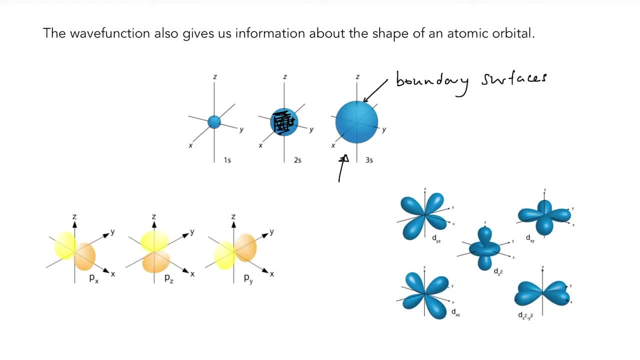 Also, we should note that as our orbitals get larger, they also become more diffuse. So when L equals 0,, then I've got an s orbital. When L equals 1,, I have a p orbital. And because the magnetic quantum number ml can be minus 1,, 0, plus 1,, that tells me I've got three different. 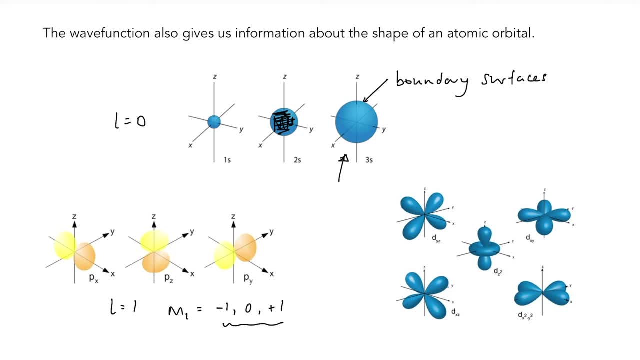 p orbitals, each with a different orientation in 3d space. So that tells me that I've got three different p orbitals, each with a different orientation in 3d space, And because the there's a quite loose now MANY reasons, that still happened At the right. but maybe, if you 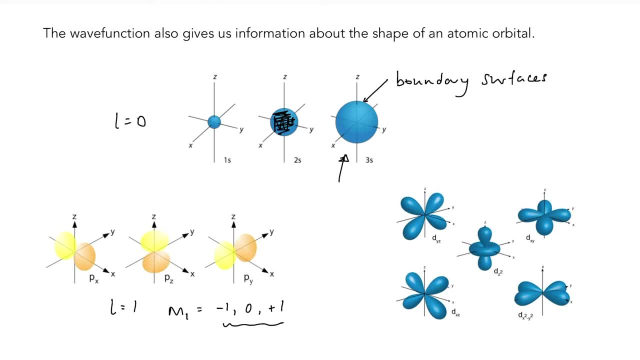 just estaban use magnificently long y. I bet you could use a point of theencias: What now? and in this picture youc and see thatquiet clearly. We know them more familiarly as the px, ry, pz orbitalsAnd when L equals 2, I've got wo numero deO produces. oh, lu, xs plus 4xs plus 8 deorbitals. 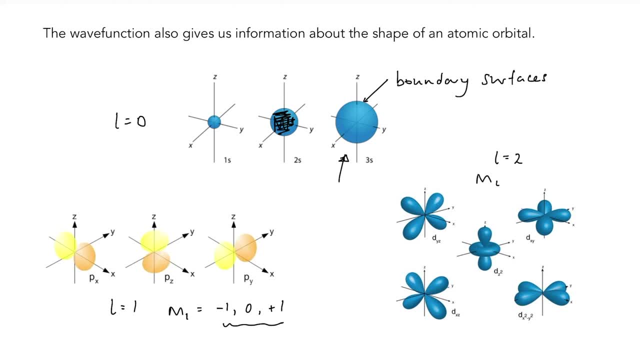 Again my magnetic quantum number minus2, then we add theSince I really didn't realize that a cube is going to be. there's less than8 odd CALSats. I'd say that's around 2d salvation zerores景ences. So if t is 0 plus 1, loosethat's plus 2 and my d orbital Coriant totals. 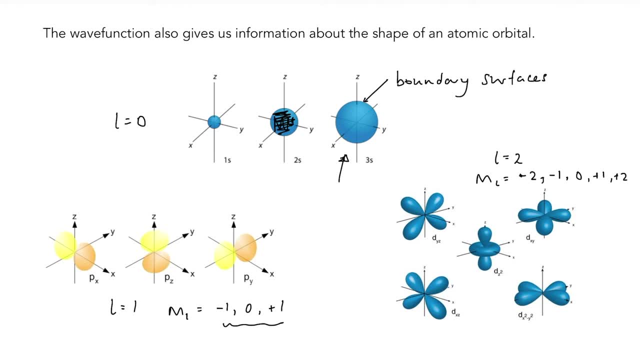 Orbitals. then we have 5d orbitals again: hu, f, forart, chains, arms us circutiQsies. Maybe we'll in 3D space. Now, as I mentioned earlier, Schrödinger's equation can't be solved, for 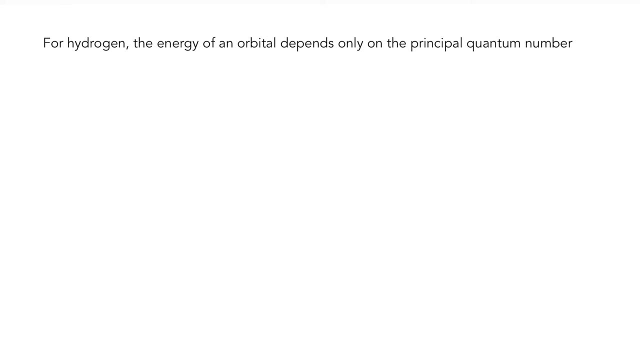 atoms other than hydrogen, But if we make a few assumptions, everything we've talked about in terms of atomic orbitals holds true for atoms with more than one electron. However, there is one very important difference between the energy levels of a hydrogen atom compared with the 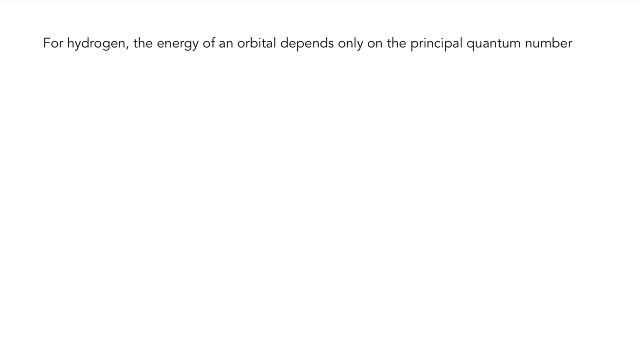 energy levels of other atoms, And this is reflected when we have a look at the atomic spectra of hydrogen in its simplicity. So for hydrogen the energy of an orbital depends only on the principal quantum number n. So for example, if we take the 2s and the 2p orbitals, 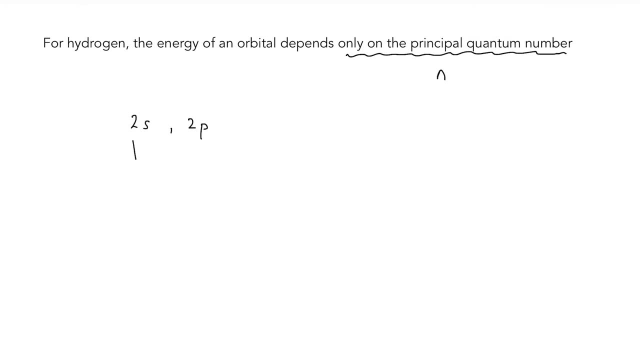 2s, 2p as an example. In each case their principal quantum number is 2, n equals 2, they both belong to that second energy level. So because the energy depends on n, they've got the same value of n. 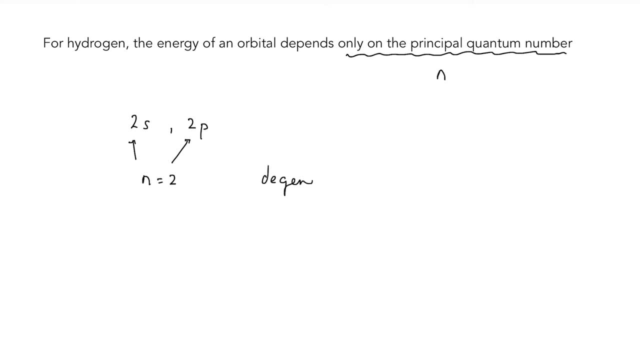 they have the same energy. They're said to be degenerate. Let's contrast that with atoms that have more than one electron. In this case, the energy of an orbital depends on l, the secondary quantum number. So let's take our 2s and our 2p orbitals. 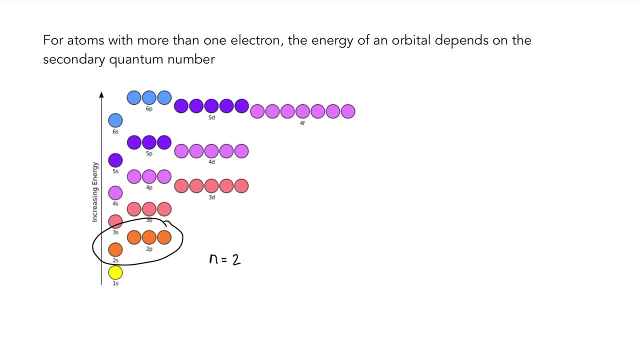 again, n equals 2, but that's not relevant here. The key here is l. For our 2s orbital l equals 0.. For our 2p orbital, l equals 1.. That tells me that the 2s orbital is of lower energy than the 2p. 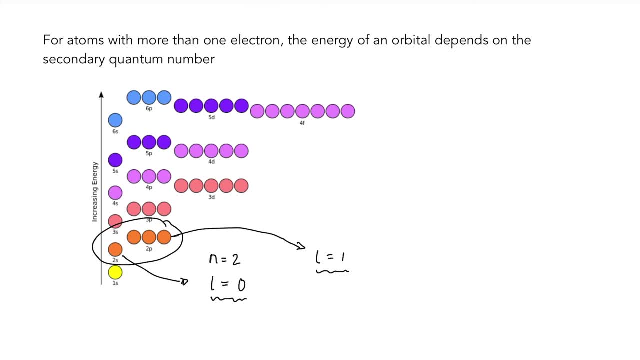 orbital. They are not the same. However, our three 2p orbitals all have the same secondary quantum number: l equals 1. So they will be of the same energy. Each of our three 2p orbitals is degenerate. 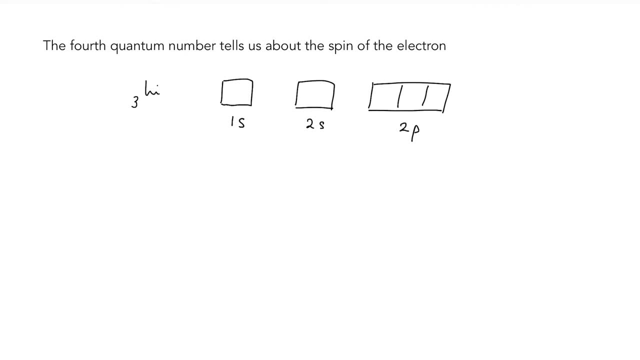 And finally, just to complete the picture, there is a fourth quantum number. and the fourth quantum number has the symbol ms, and it tells us the spin of an electron. An electron can either be spinning clockwise, in which case ms equals plus a half. 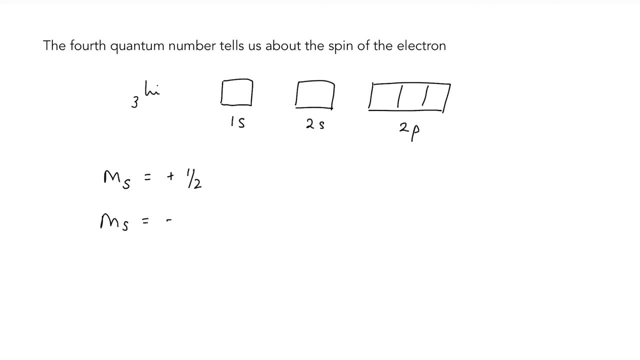 half or anti-clockwise, in which case ms equals minus a half, And once again we've represented this in terms of doing electron configurations for atoms or ions. Lithium, for example, has got three electrons. We know that the first two are going to go into the 1s orbital and our electrons. 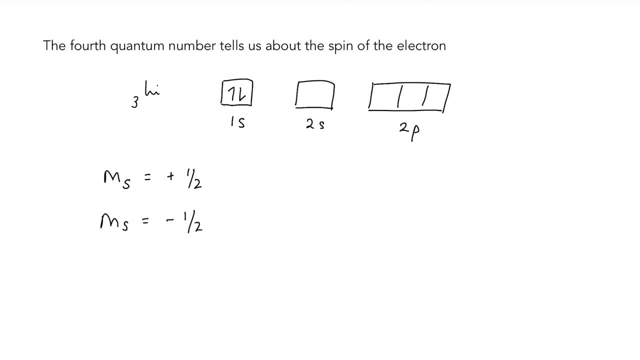 are going to be spin paired. One is going to be spinning clockwise, one anti-clockwise to minimize the repulsion between them, And of course the third electron would go into the 2s orbital. So I hope that that clears up a little bit of the background theory behind where we get our